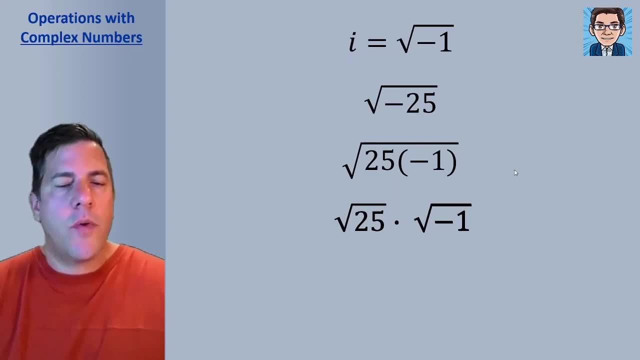 So the square root of 25 is 5, but then the square root of negative 1,, as we've defined, is i, and then the answer to this becomes 5i. So it allows us to take the square root of a negative number. 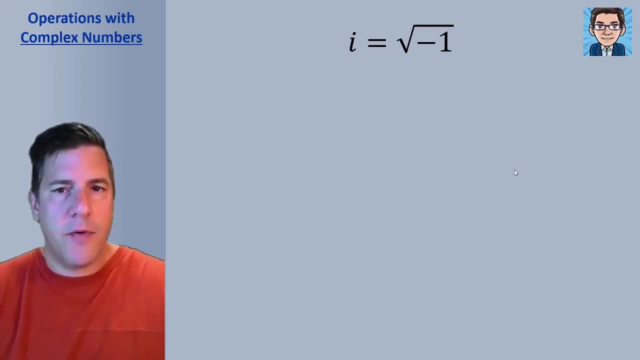 Now, an important concept when you're doing operations with complex numbers is i squared. So if i is the square root of negative 1, then i squared is going to be the square root of negative 1 times the square root of negative 1,, which just ends up being negative 1.. 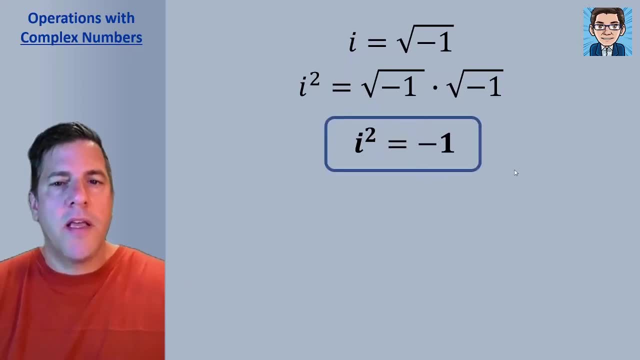 So a very important concept when we're doing operations with complex numbers is that i squared is negative 1.. So whenever we're doing operations, we treat a variable i just the same as any other variable. So if we had 5i plus 10i, we would get 15i. 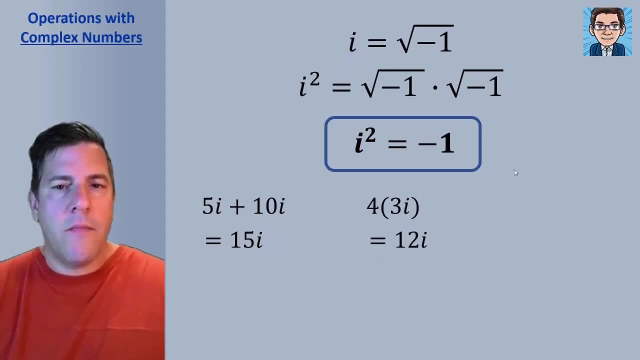 Four times 3i, we would get 12i. Okay, But when we get a case like this, 6i times 5i, we'd get 30i squared. but rather than a regular variable, we've got to go one more step now, because the i squared is equal to. 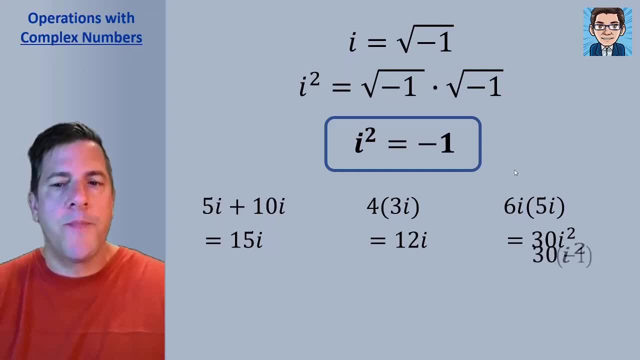 negative 1, so we've got to replace the i squared with negative 1.. And this becomes 30 times negative 1, or just negative 30.. Okay, let's take a look at how to simplify something. So if we have i in the denominator, 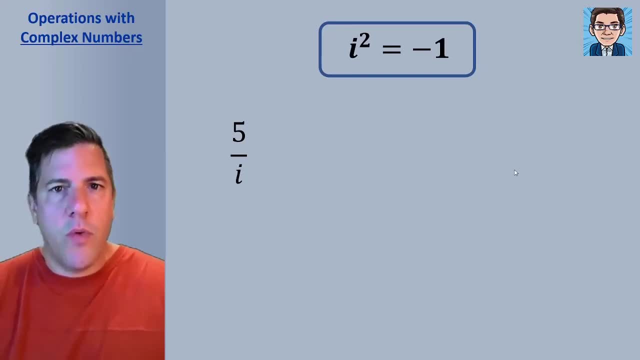 Since i is defined as a square root, we can't have a square root in a denominator to have something fully simplified. So 5 over i. we can simplify that by multiplying both the numerator and denominator by i. So if we multiply the numerator and denominator by i, we're multiplying by 1.. 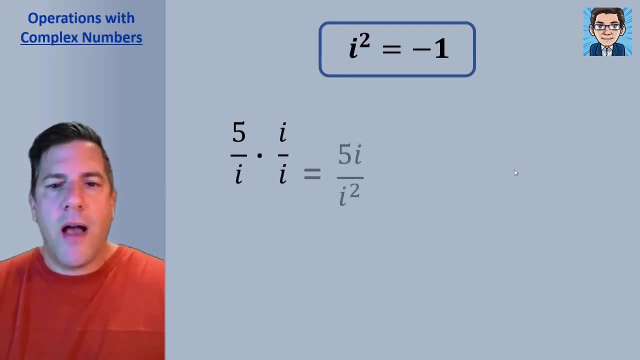 So we can do that. So the numerator is going to be 5i and the denominator is going to be i squared, And again we need to know that i squared is negative 1, and we're going to replace i squared with negative 1.. 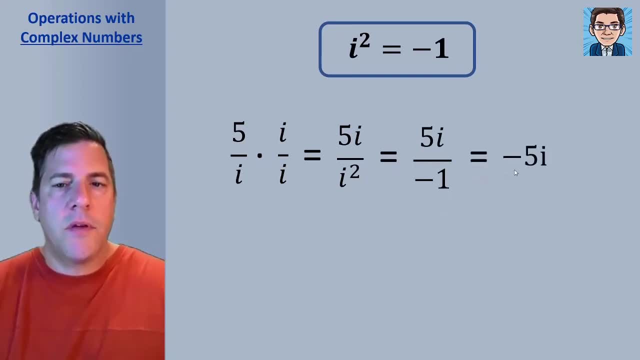 So then, 5i over 5i, Okay, Okay. So 5i over negative 1 just becomes negative 5i. Now if we have a more complicated, where we've got that was just an imaginary number in the denominator. 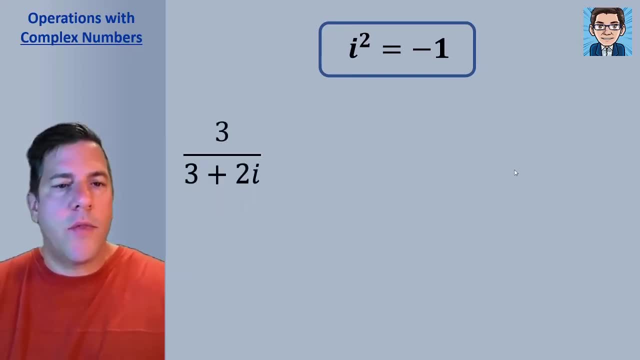 What if we have a complex number in the denominator? How would we simplify 3 plus 2i? Well, we're going to multiply it by something that's called the conjugate. So the conjugate of 3 plus 2i is going to be 3 minus 2i, and you'll see why we chose. 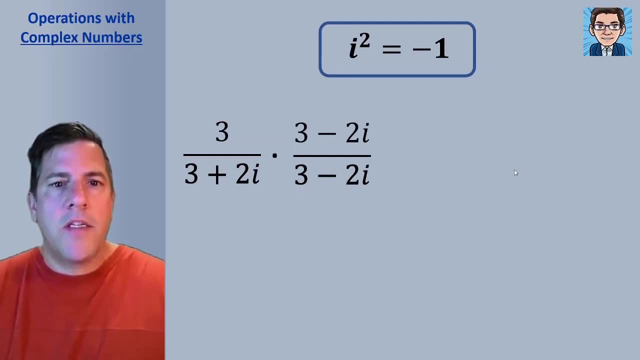 that particular thing in a second, And it's just because that's going to help us cancel out. so we have no more imaginary number in the denominator. Let's see how that's going to work. So if we multiply the numerator, the 3 times the 3 is 9, and the 3 times the minus 2i is. 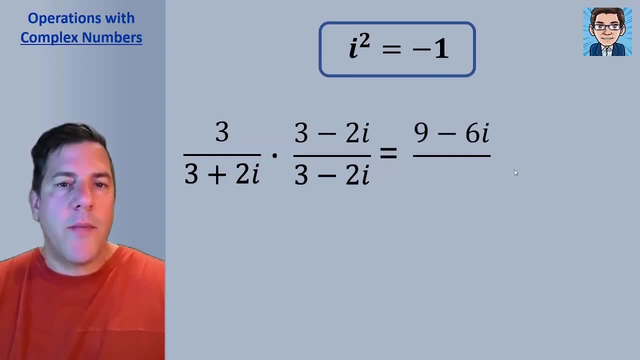 going to be minus 6i. But let's take a look at what we do with the denominator. So the denominator, we've got to multiply 3 plus 2i and 3 minus 2i. So let's multiply this out by FOIL. 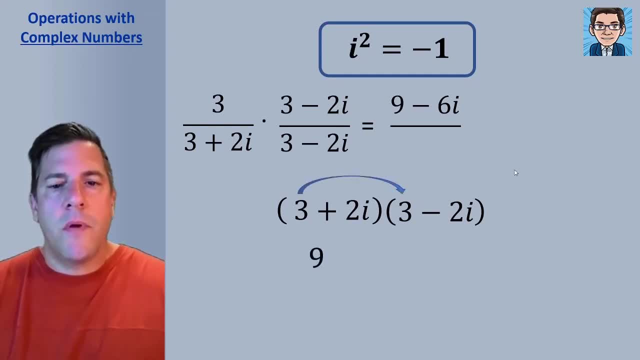 The first 2 is going to get us 9.. The last 2, I mean the outers- is the 3 times the minus 2 is going to get us minus 6i. The inners, the 2i and the 3, is going to get us plus 6i. 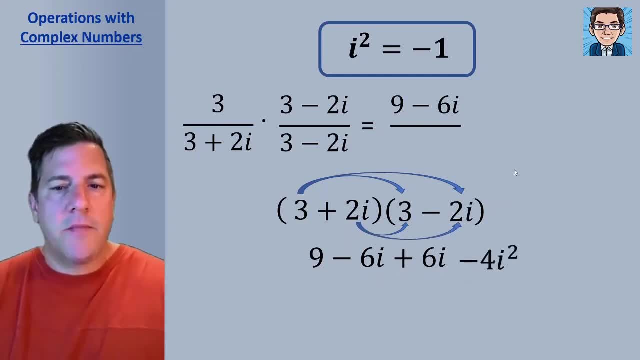 And the last 2, the 2i and the minus 2i is going to get us minus 4i squared. Now, when we do the math here, the minus 6i and the plus 6i cancel out and those middle. 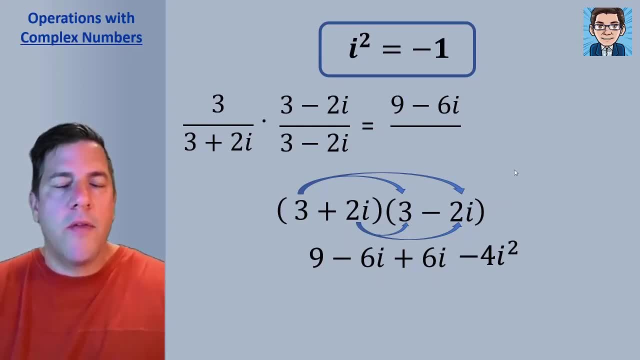 two terms are always going to cancel out. when we pick a conjugate, when we pick the same two terms, When we pick a different sign, those two middle terms are going to be the same, except with different signs, and they're going to cancel out. 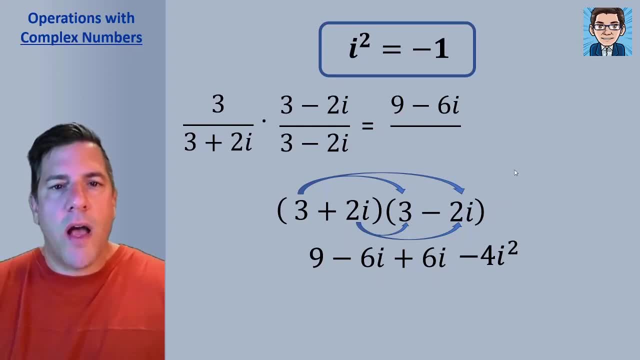 So those two are going to cancel out. we're just going to be left with 9 minus 4i squared, But we're going to replace that i squared with negative 1.. So this becomes 9 minus 4 times negative 1, or 9 plus 4, or 13.. 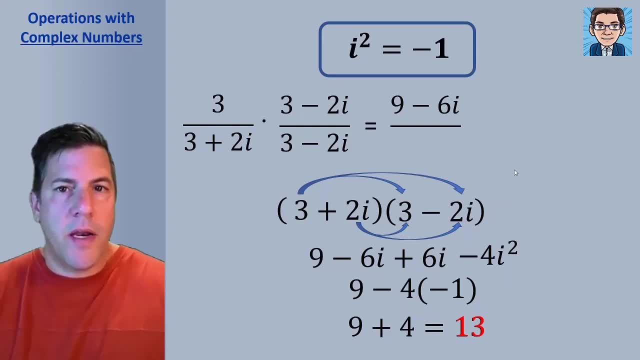 So that whole denominator now has no imaginary number in it anymore, So it's just a whole number. So that denominator, That denominator is 13,. and then, to do the final step, to simplify this, we just split it up into two parts: the 9 over 13, and the minus 6 over 13i. 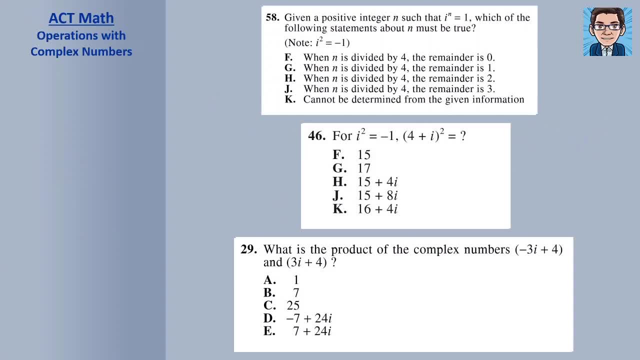 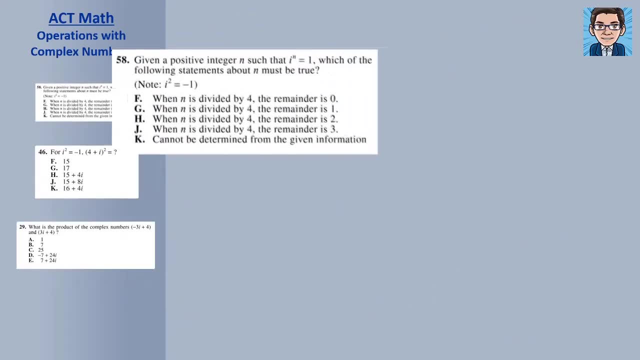 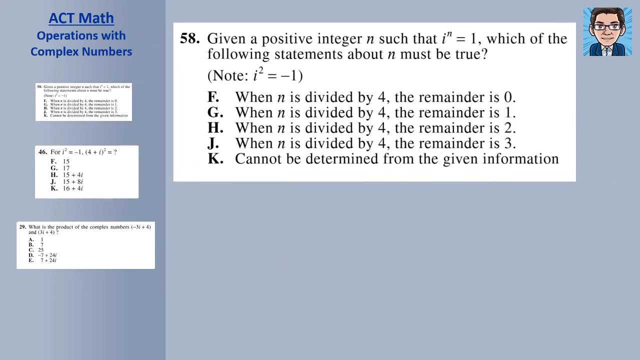 Okay, I've got three practice ACT math problems that have to do with complex numbers. Let's take a look at this first one. So this first one is saying that a positive integer n- we have i to the n- equals 1.. So which of the following must be true? 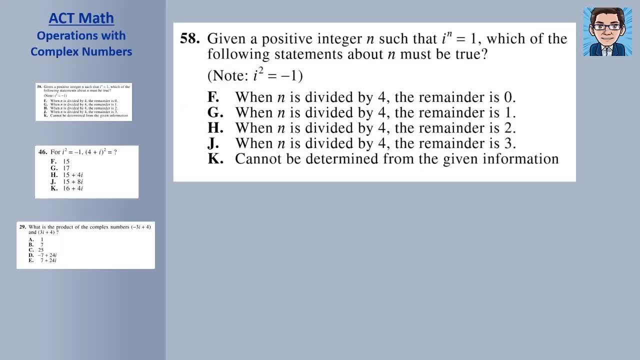 So let's take a look. So it tells you that i squared is negative 1, so that's helpful. So i to the first power is just i. i squared, which we talked about, which they also give you right here, is negative 1.. 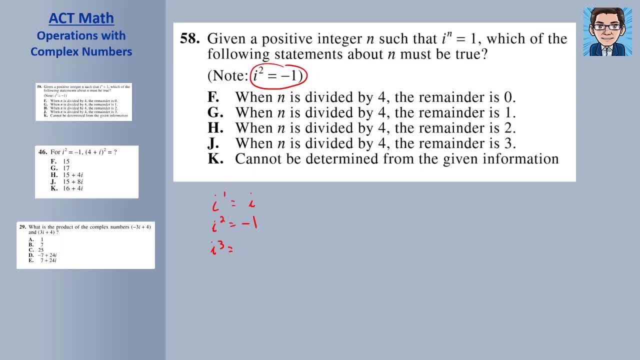 i to the third. power is just going to be i to the first times, i to the second, or i times negative 1.. i to the fourth is going to be: i squared times. i squared or negative 1, times negative 1, or positive 1.. 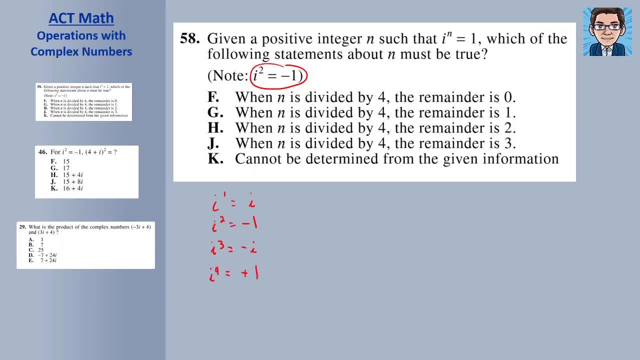 And then the pattern repeats after this, Because i to the fourth is 1,. any time you have a multiple of i's, four of them are going to make 1.. So it's just 1 times this, so we can take out multiples of 4.. 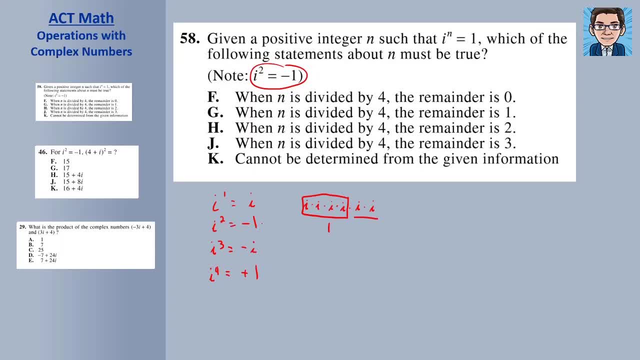 And then the value of this is just going to be i squared, which in this case would be negative 1.. So let's go back to the problem. So it's telling us that the value is going to be 1.. So if we divide by 4, what does the remainder have to be for us to be 1?? 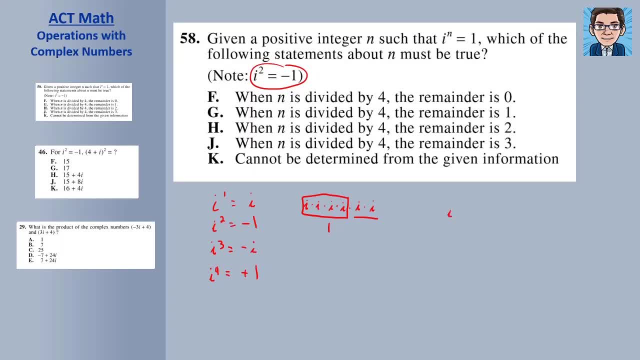 So we have all these groups of 4.. If we have one, i left, In other words, the remainder. If the remainder is 1, it's just going to be i. If we have 2 i's left, it's going to be negative. 1, i squared. 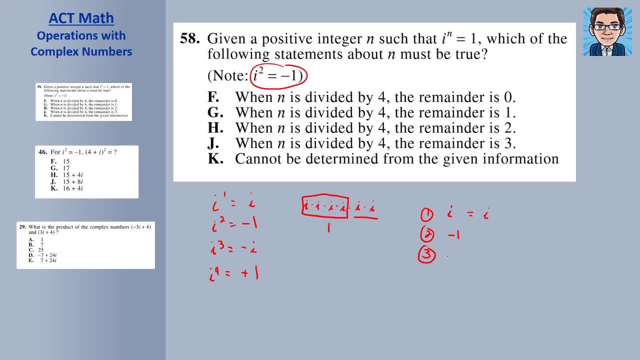 If we have 3, the remainder is 3, it's going to be negative i And if the remainder is 0, then we just have multiples of 4 i's, which is just going to be 1 times 1 times 1.. 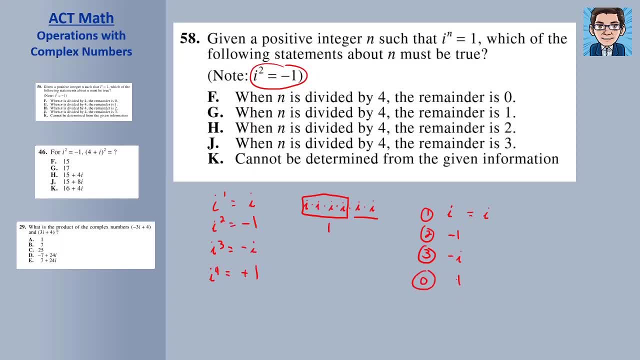 So if we have 0 left, the value is going to be 1.. So if we know that i to the n equals 1., Then if we divide by 4, any set of 4 i's multiplied together is going to be 1, and 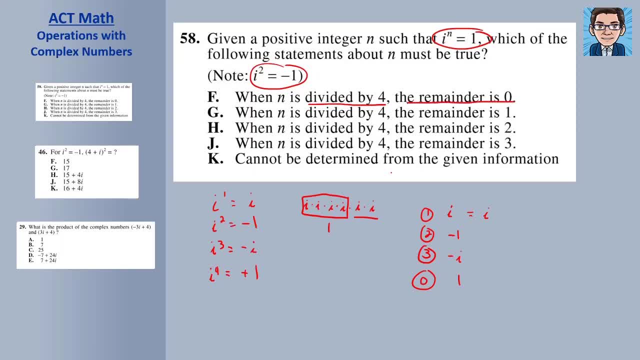 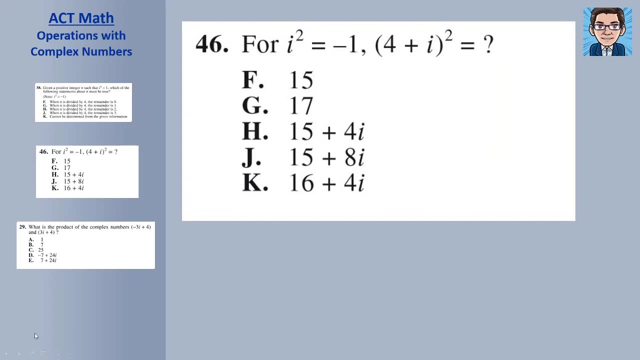 the remainder is 0.. So this first one is going to be our answer. That's going to get us a number that equals 1.. Okay, on the second problem, we're doing 4 plus i squared. Let's just write that a different way, right? 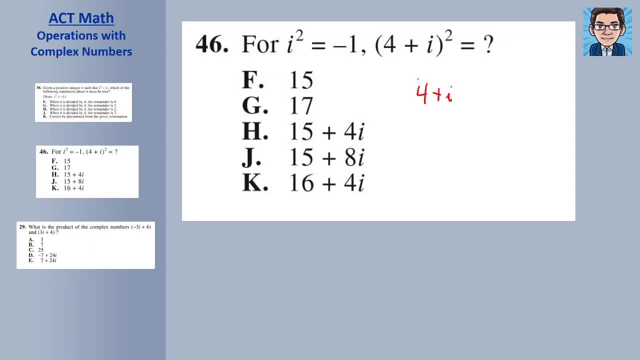 So let's just write that as 4 i squared. Okay, 4 plus i times 4 plus i. it might just be a little easier to see. Then multiply it out by FOIL: 16 plus 4, i plus 4, i plus i squared. 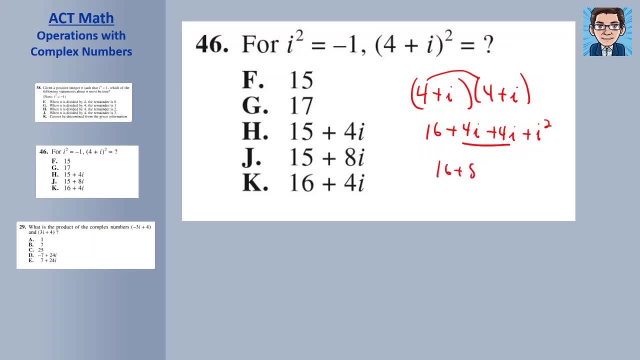 Combine our like terms 4 i and 4 i is 8 i. Here they tell you this: i squared equals 1.. The SAT usually doesn't tell you that, but the i squared equals negative 1.. So we can replace i squared with negative 1 and get 16 plus 8 i minus 1.. 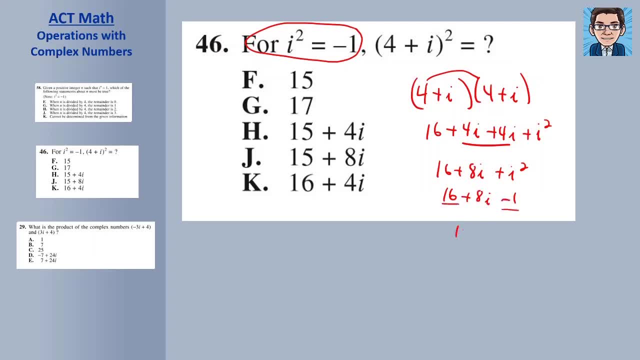 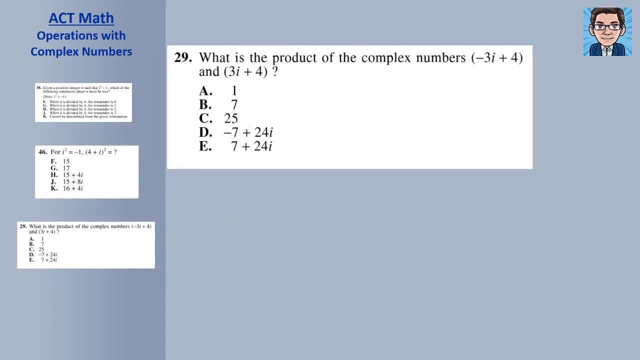 Then combine our like terms: the 16 and the minus 1 is 15 plus 8 i, and that matches our answer right there for j. All right, and the third problem: we're going to multiply negative 3 i plus 4 times 3 i plus. 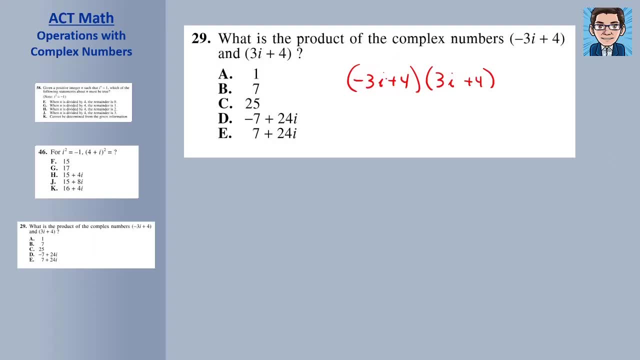 4. And again, let's multiply it out. Negative 9 i times I mean negative 3 i times 3 i is negative 9, i squared. We're going to get minus 12 i and plus 12 i. 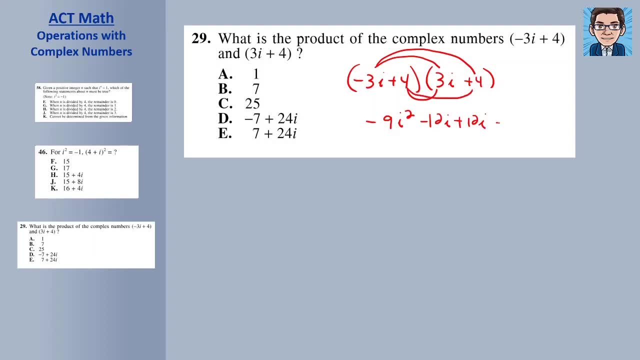 Okay, And then the 4 times 4 is going to get us 16.. Now the minus 12 i and the plus 12 i are going to cancel each other out And we're just going to get minus 9, i squared plus 16.. 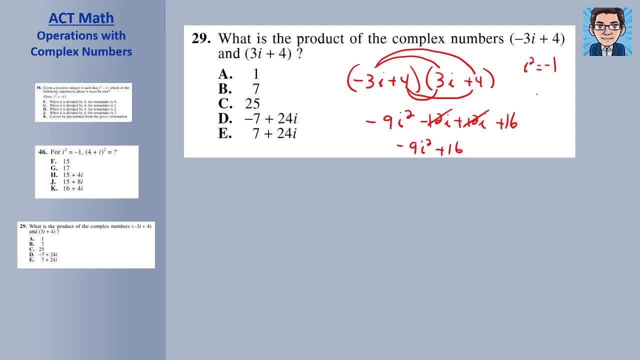 We know that i squared is going to equal negative 1.. So we've got to replace this i squared with negative 1.. So we're going to get negative 9 times negative 1 plus 16.. which is 9 plus 16, or 25 is our answer, which matches answer C. Now notice that. 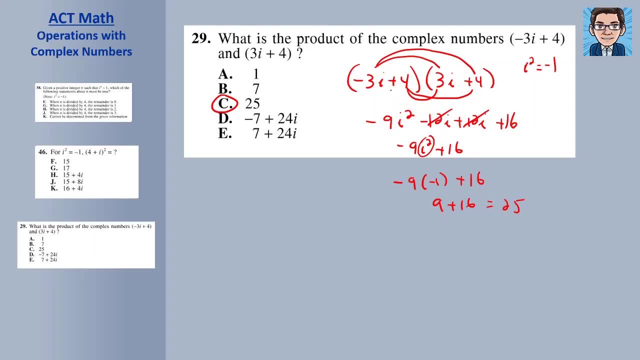 the i's cancelled out. It might not have been as apparent here that this is a conjugate, but it's just rewritten the other way. So this is just the same as 4 plus 3i and 4 minus 3i flipped around, right? So it's just a conjugate, That's. 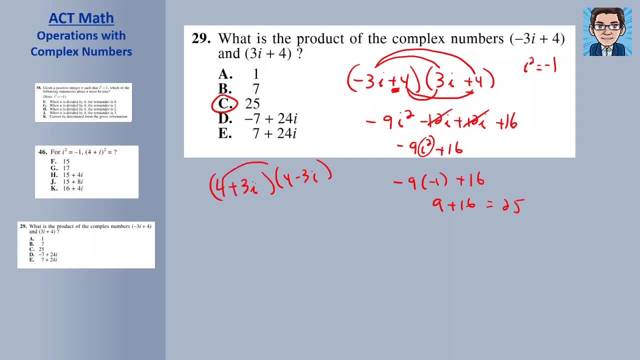 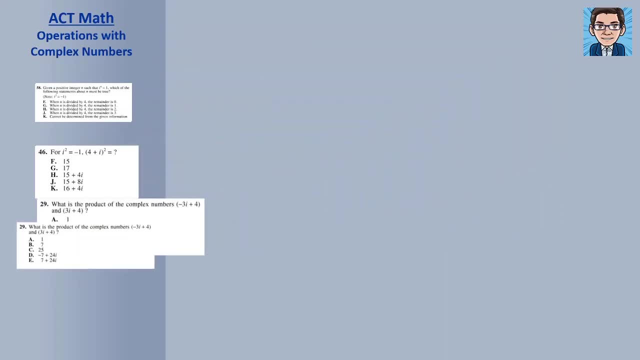 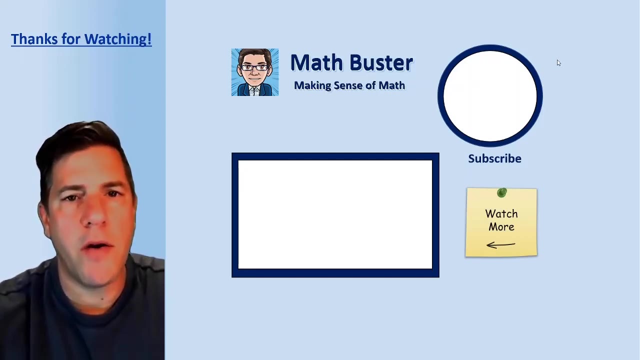 why we get the middle terms cancel out and we get: 16 plus 9 is 25.. Thanks for watching. If you have an ACT test coming up, good luck with it. If you're new here and you'd like to subscribe, you can do so right over here. I've got other 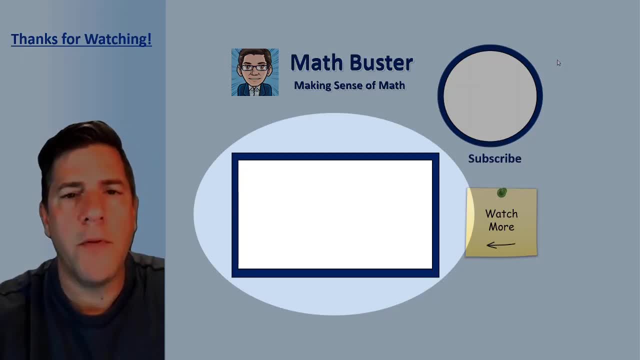 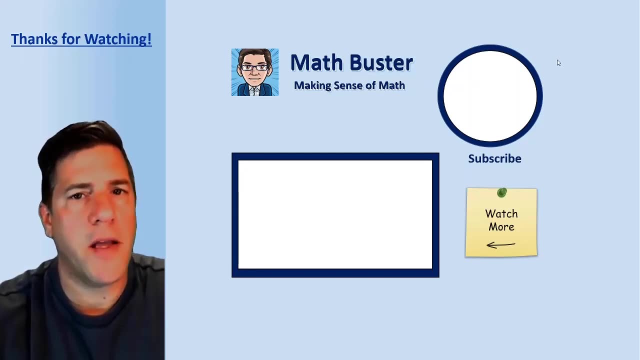 suggestions of videos for you to watch right here. Please comment below on things that you liked about the videos or ways that I can improve it, And thanks for watching And come back again soon.